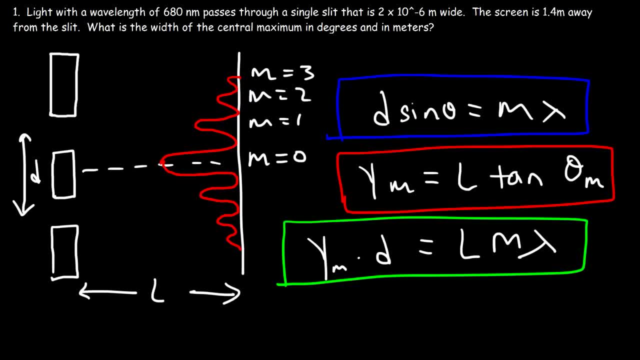 only if theta is small. Now, as d decreases, theta increases. So if the width of the slit is like very small, you need to be careful, because if the angle is large, then this equation doesn't work. So in this example, d is very, very small. So if the width of the slit is 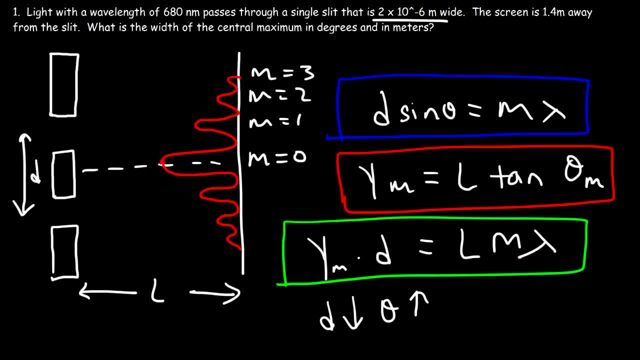 very small. we're not going to use that equation, But if d was like, let's say, 5 millimeters, that's large enough, where theta will be very small, and we could simply use that formula: That's theta 1, and here we have theta 2, and so forth. So you know what the angles. 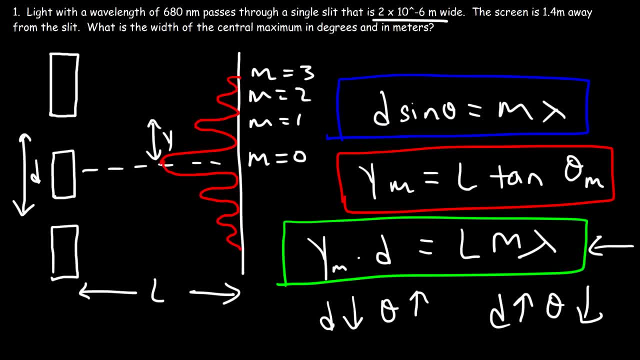 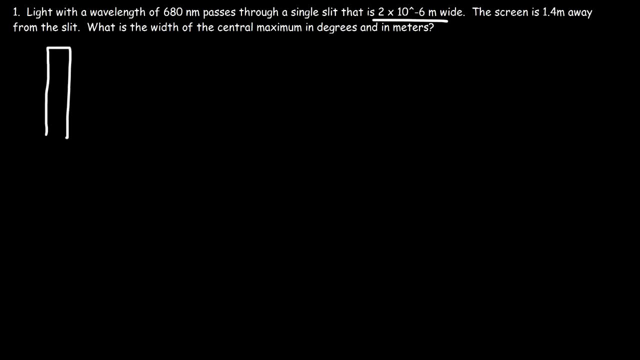 are. This is y1, with the first bright fringe, and this is y2.. Now let's talk about the single slit experiment. So instead of two openings, there's going to be only one opening, And this is going to be the screen. Let's tell the distance. 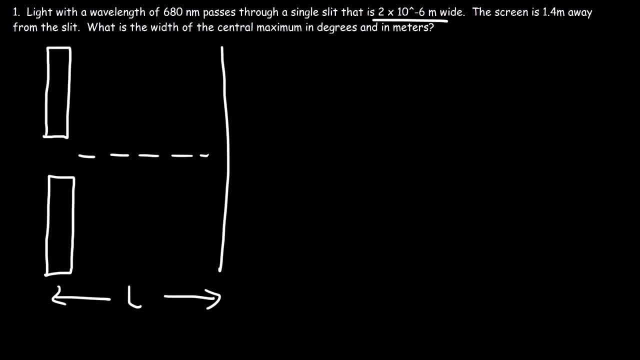 between the screen and the other side. So this is the width of the slit, which is d, and the pattern is going to be different. In the middle we're still going to have a very bright fringe And then after that there's not going to be any significant bright fringes anymore. 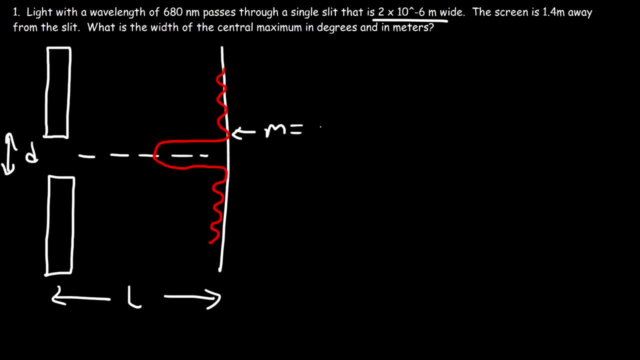 So at the first dark fringe, that's where m is equal to 1, and here m is equal to 2, and then here m is equal to 3.. m is based on the dark fringes or where destructive interference occurs. 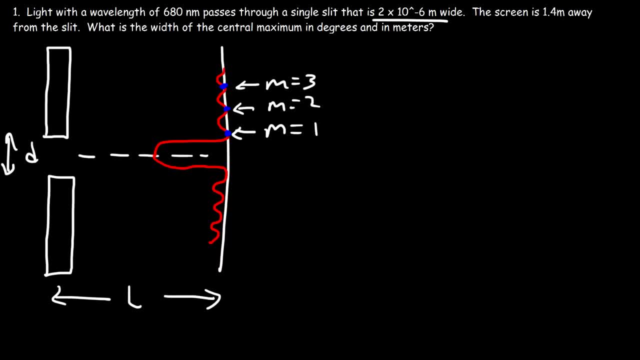 So now let's focus on this problem. What is the width of the central maximum? in degrees and in meters? So this is the central maximum. So we need to calculate this width right here. So let's focus on the top triangle. This here is y1.. y1 is the distance between the center. 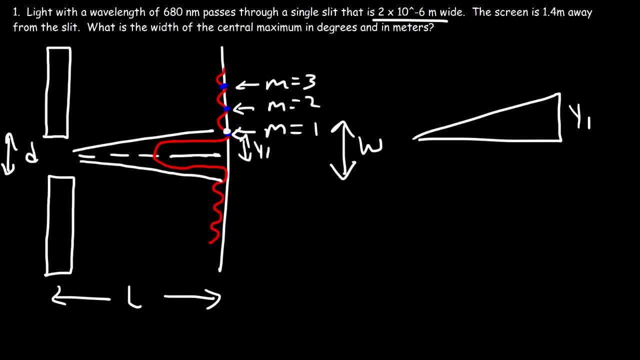 and the first dark fringes. So that's y1.. So the width that we're looking for is basically twice the value of y1.. So this is the width that we need to calculate. That's going to be in meters. Now we also want the angle of the central maximum. 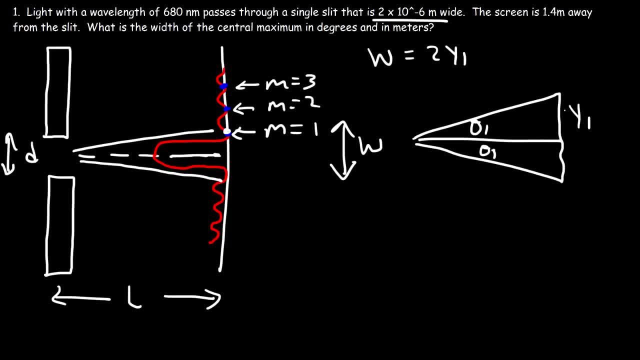 So let's say, this is theta 1.. So the angle that we want is really this total angle, or 2 theta 1.. So that's y1.. So that's y1.. So that's going to be the angle of width, so to speak. 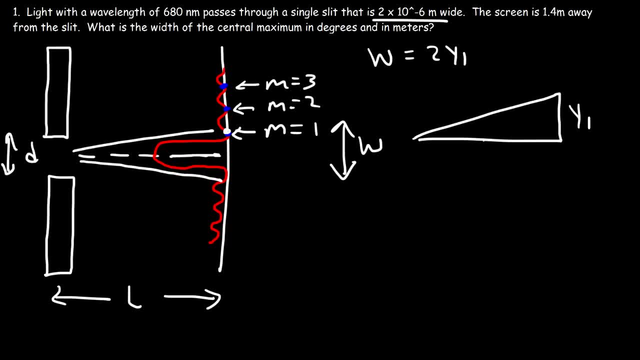 So if we can calculate theta 1, we can calculate all of it. So let's focus on finding theta 1, and this is L. So first let's use this equation: d sine theta is equal to m times lambda, So d is 2 times 10 to the minus 6.. 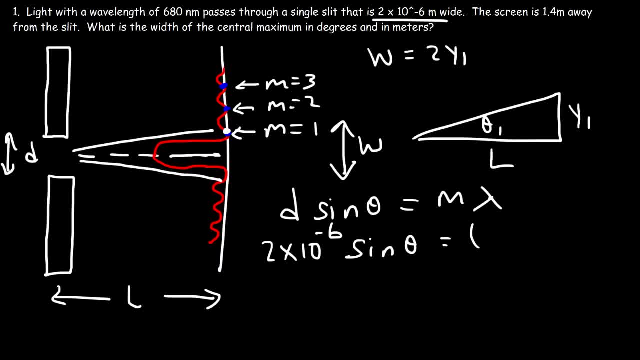 m is 1 for the first dark fringe And lambda is 680 times 10 to the minus 9 meters. So if we take 680 times 10 to the minus 9 and divide it by 2 times 10 to the minus 6,, 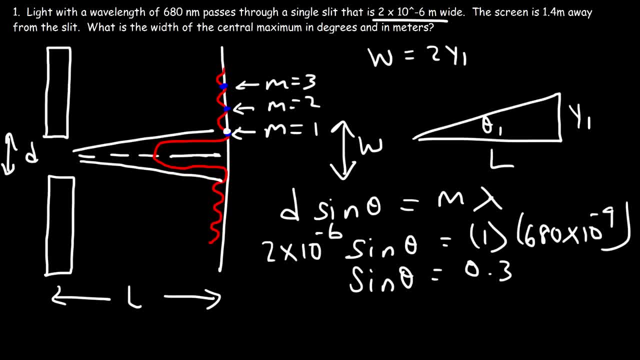 we can see that sine theta is 0.34. So theta is going to be the arc sine of 0.34. And so theta 1 is 0.34. 0.34. 0.34. 0.34.. 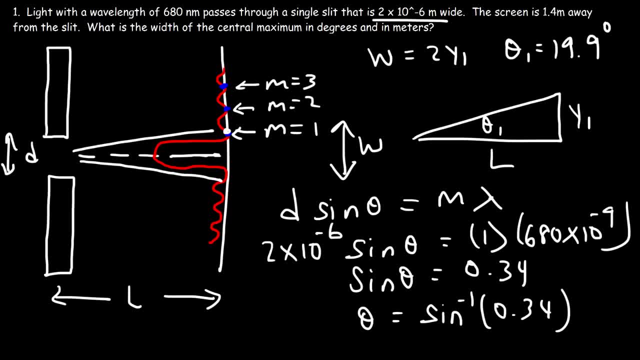 0.34.. 0.34.. 0.34.. 19.9 degrees if you round it. So that's a fairly large number. So we can't use that third equation where theta is small. So the angular width or the width of the central maximum in degrees is twice this. 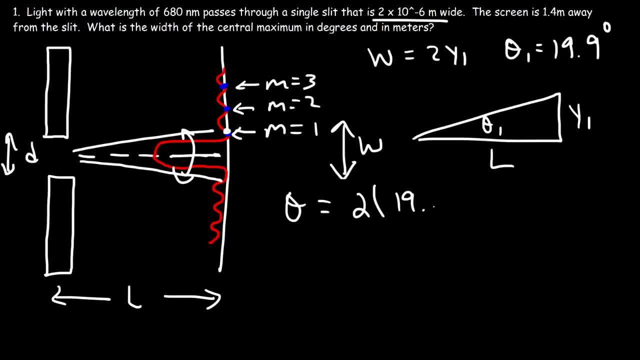 value. Now, the exact answer was like 19.877,. for those of you who don't want to round it, The third equation of theta was 2.58. 2.58. 2.58. 2.58.. 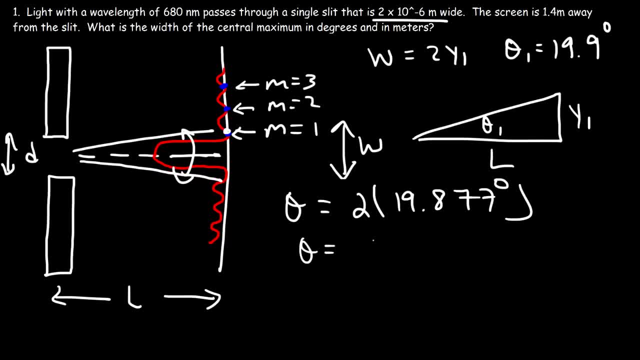 2.48., 2.48., 2.48., 2.48., 2.48.. so the angular width is 39.75 degrees, and so that's the answer to the first part of the problem. now let's move on to the second part. so we need to calculate. 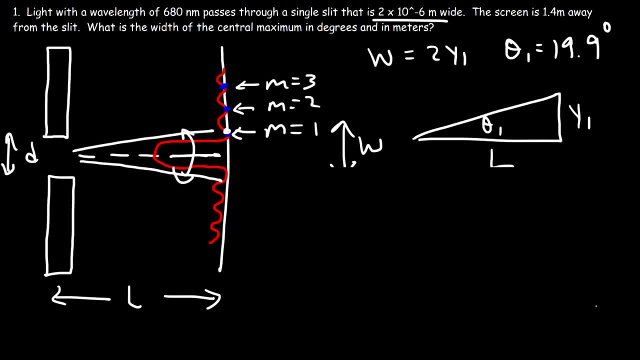 y1. so we can use this equation: y sub M is equal to L tangent theta M. so we're looking for y1. L is 1.4 meters and we need to use theta 1, which is nineteen point eight, seven, seven degrees. so y1 is about point five, zero, six, two meters, and 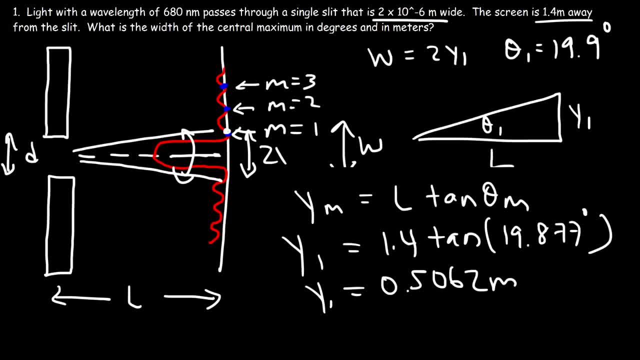 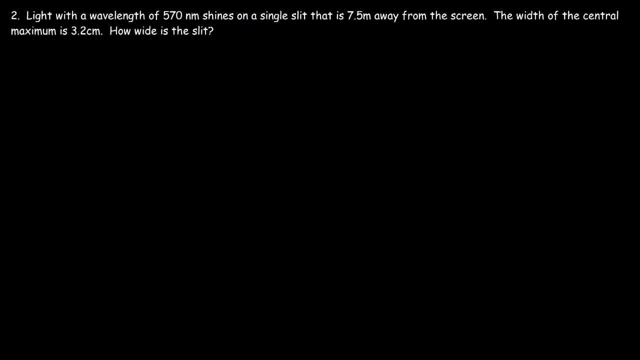 so this entire width represents 2y1. so the width is going to be 1.01 meters, and so that's the width of the central maximum. that's the answer to the second part of the problem. let's work on another problem. light with a wavelength of 570 nanometers shines on a single. 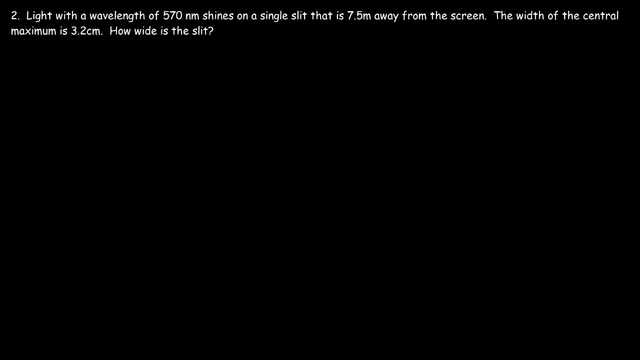 slit that is seven point five meters away from the screen. the width of the central maximum is three point two centimeters. how wide is the slit? so let's start with a picture. so we have a single slit. let's say this is a screen and so this is L and this is D. 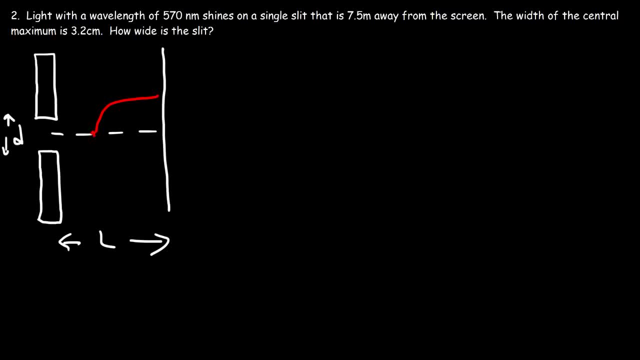 and let's say, this is the central maximum, you, so our goal is to calculate D. now we have the width of the central maximum, so this right here is 3.2 centimeters, and we draw a triangle, which I'm going to redraw here. this is y1 and this is L and this is theta 1, so the width of the 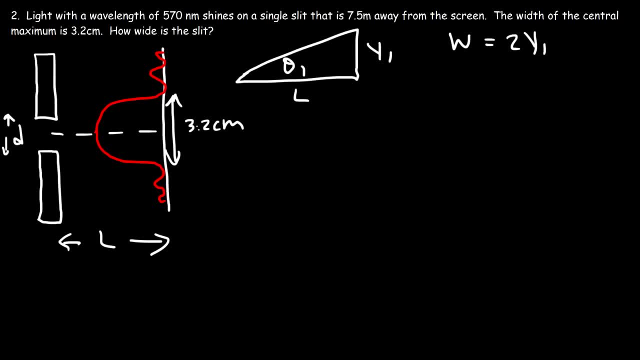 central maximum is twice the value of y1. So this is W and this is Y1, so you can visually see it. Now let's make a list of what we know. So Y1 is half of W. so 3.2 divided by 2, that's 1.6 centimeters. 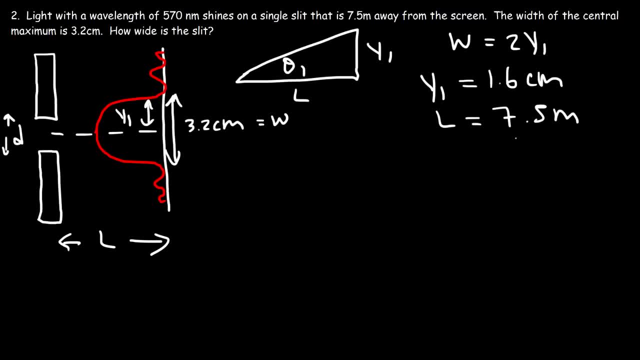 We have L, which is 7.5 meters. We have lambda, that's 570 nanometers. We don't know the angle and we don't know D, So let's calculate the angle first. So let's use this equation: Y1 is equal to L, tangent theta 1.. 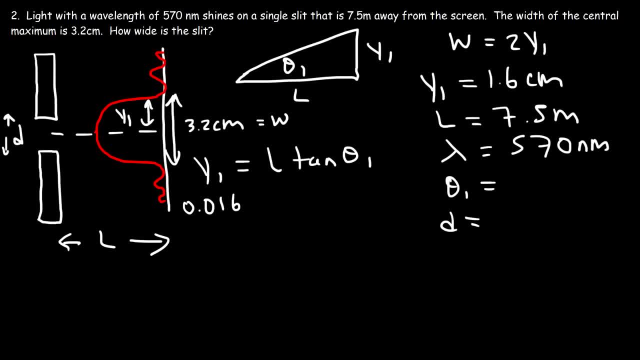 So Y1 is 1.6 centimeters, which is 0.016 meters, L is 7.5 meters, And so 0.016 divided by 7.5, that's equal to 0.002133 repeated. 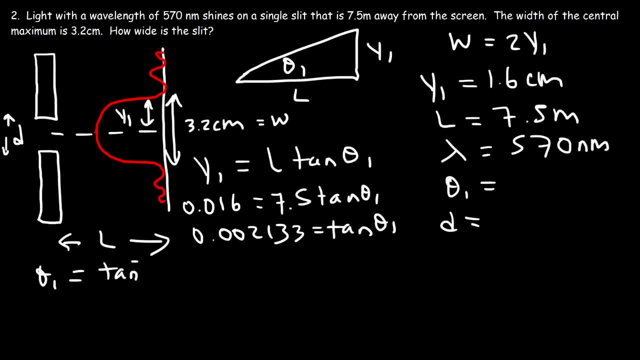 And so the angle is going to equal arc tangent. And so the angle is going to equal arc tangent of this value. So the angle is small, it's 0.122 meters. So now that we have the angle, we can calculate D using this formula. 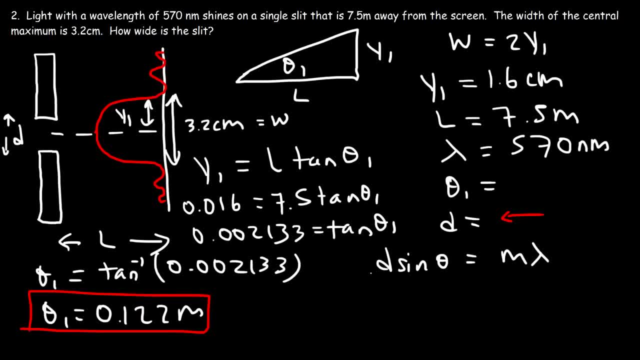 D sine theta is equal to M times lambda, So this is going to be sine of that angle, 0.122.. And M is 1, because we're dealing with the central maximum only. So here the first dark fringe will have a value of 1.. 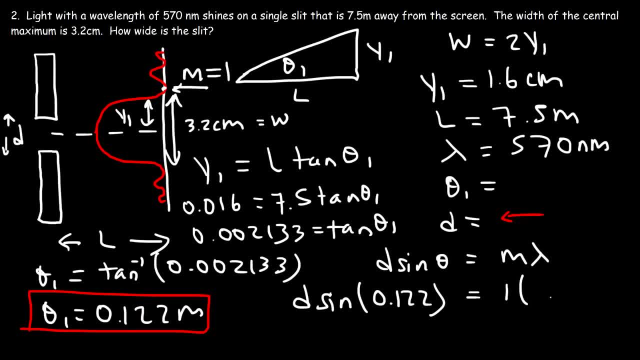 And lambda. that's 570 times 10 to negative 9.. So it's 570 times 10 to negative 9, divided by sine of 0.122.. And so in this example, D is 2.68 times 10 to the negative 4 meters. 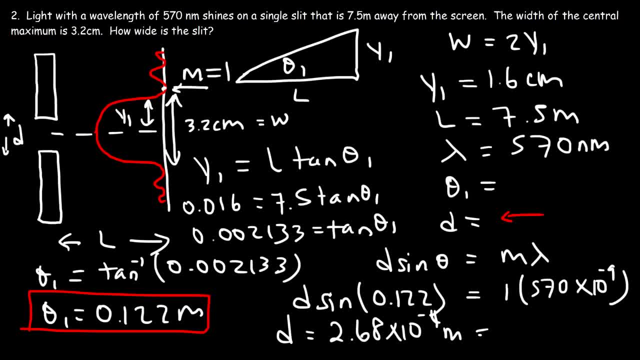 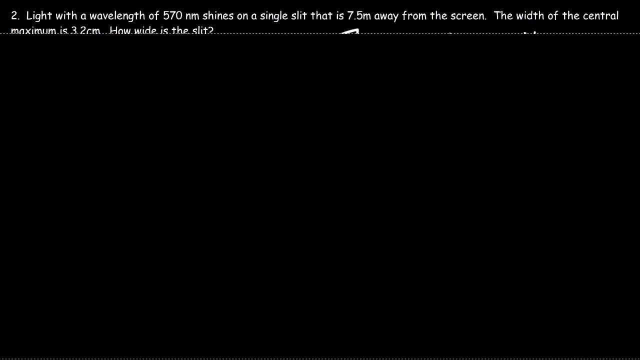 So if we divide that by 10 to the minus 3, that's about 0.268 millimeters. Now let's see if we can get the same answer using that other formula, since theta is very small, And so that's this formula.